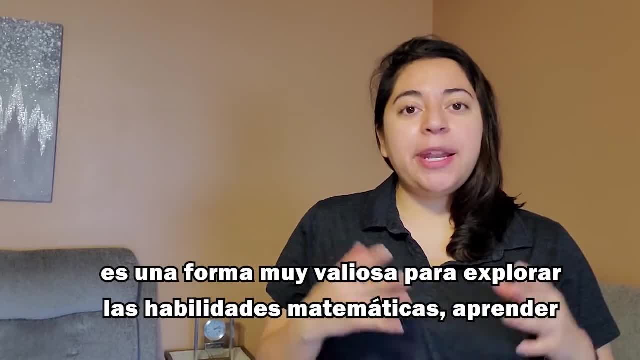 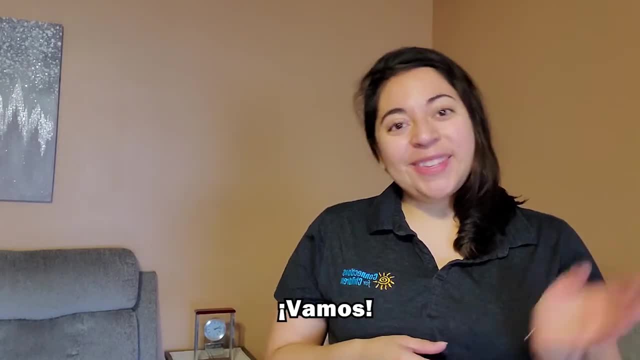 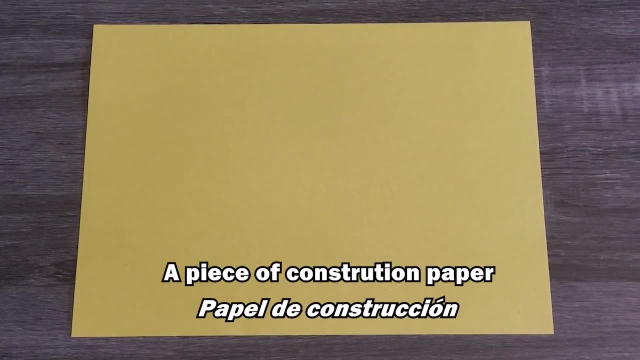 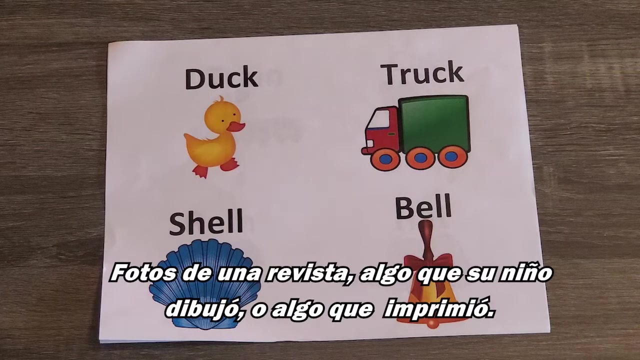 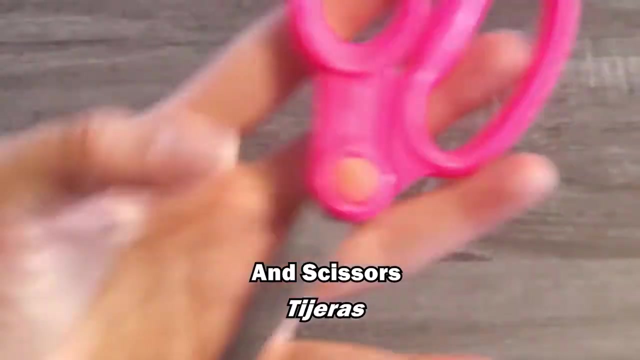 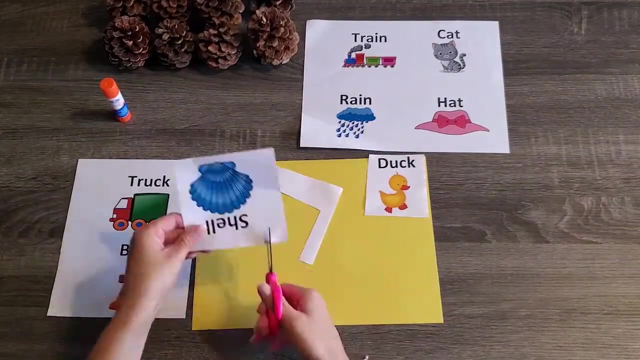 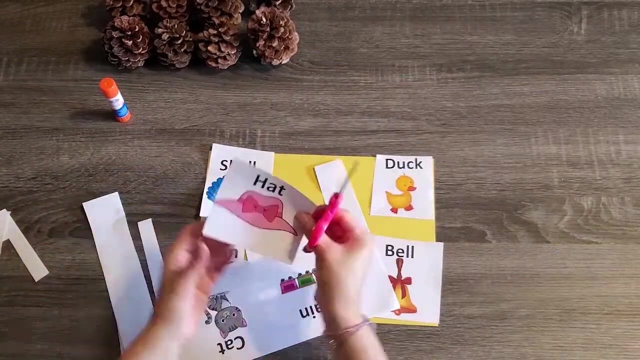 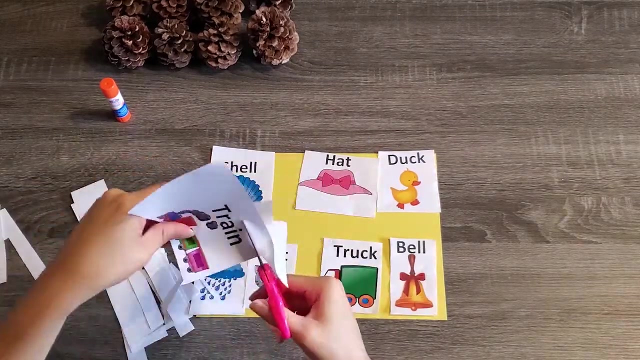 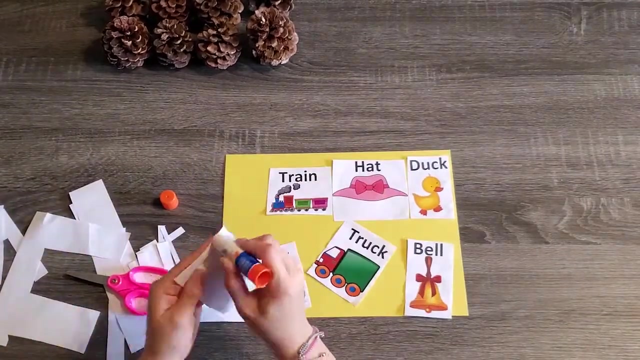 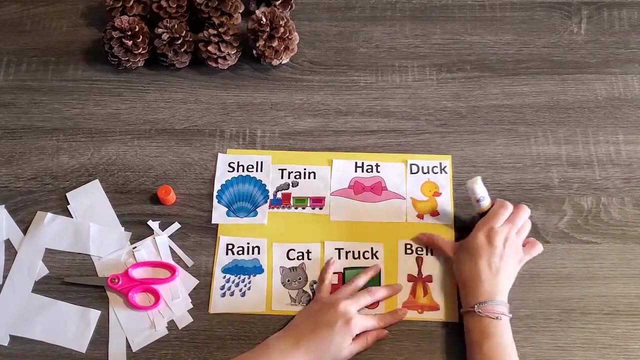 For this activity you're going to need a piece of construction paper, pictures from a magazine, something your child drew or just something you printed- glue and scissors. Tijeras, Let's get started Now. we can rhyme some words. A quick tip to remember Words that. 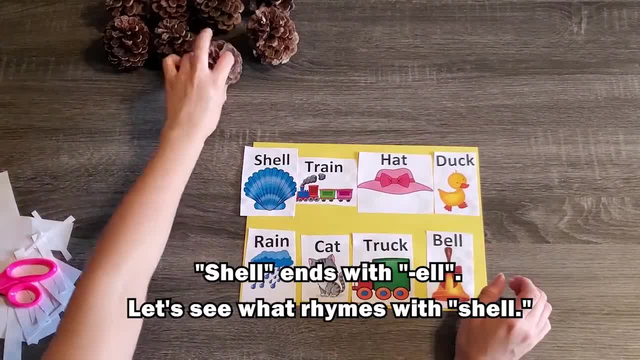 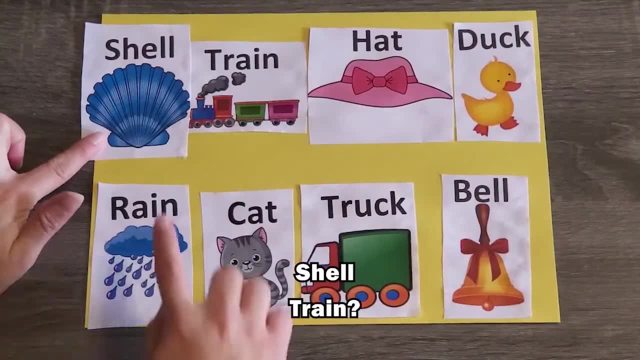 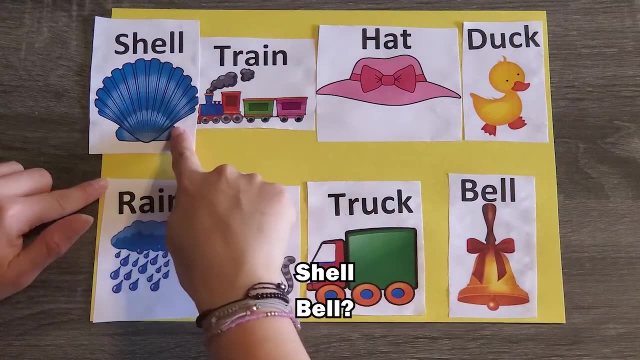 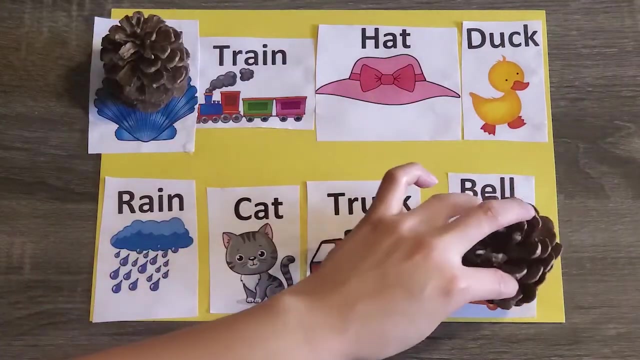 rhyme end with the same letters. Let's see Shell ends with e-l-o. Let's see what rhymes with shell, Shell, Shell train No, Shell duck, No, Shell, Bell. Yes, shell and bell rhyme. How about train? 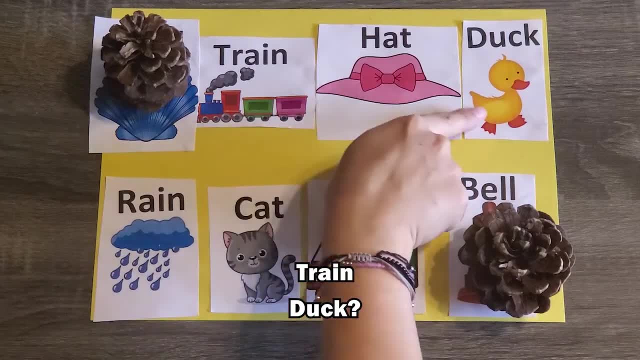 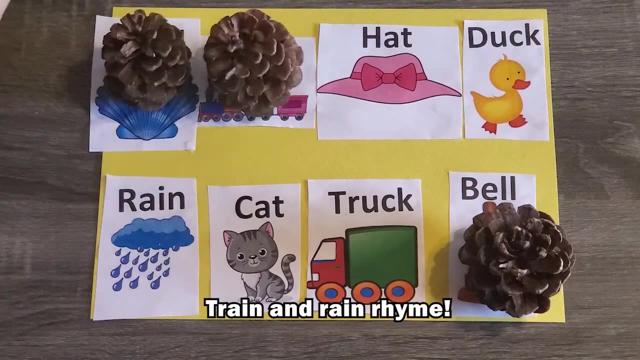 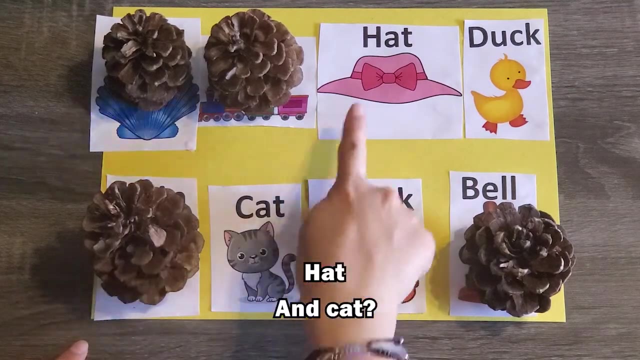 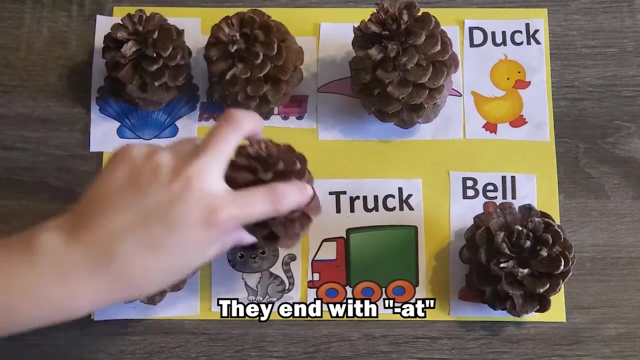 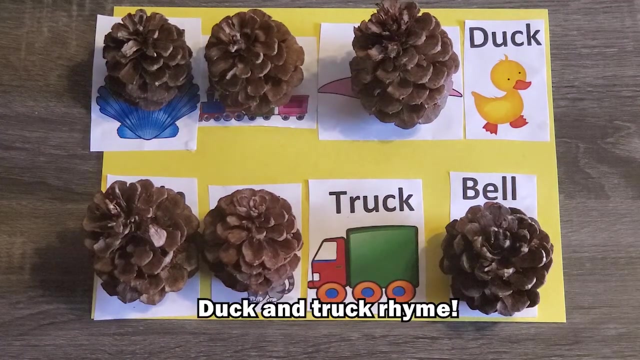 Train hat: No, Train duck: No, Train rain, Yes, train and rain rhyme. Hat and duck: No. Hat and cats: Yes, hat and cats rhyme. They end with A-T And duck and truck. Perfect, duck and truck rhyme. 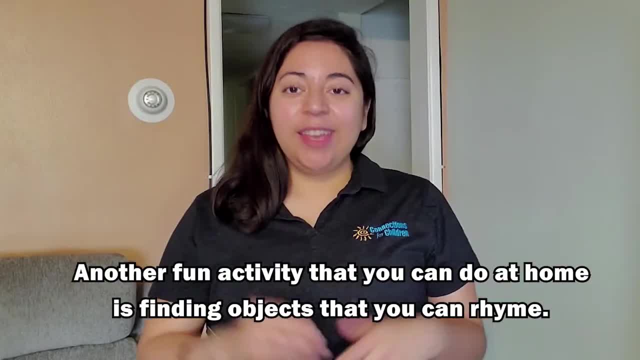 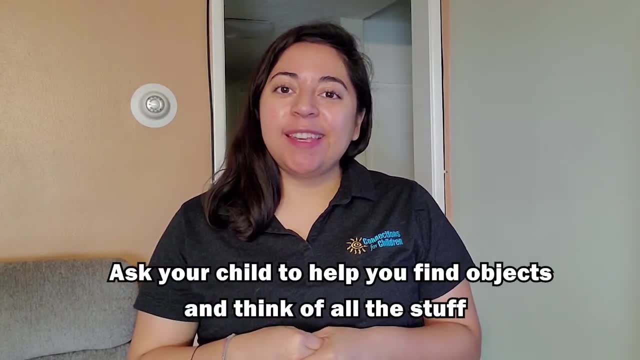 Good job everyone. you did great. Another fun activity that you could do at home is finding objects that you can rhyme. Ask your child to help you find objects and think of all the stuff that can rhyme with it. Today, my friend Riley and Benjamin are gonna help me along. 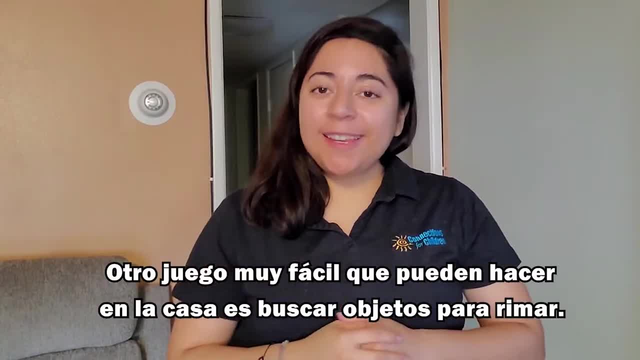 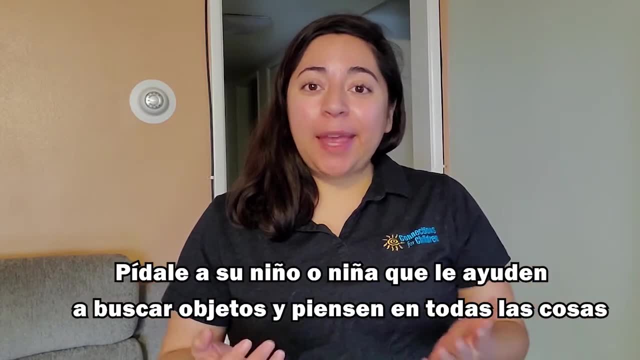 to find objects that we can rhyme at home. Otro juego muy fácil que pueden hacer en la casa es buscar objetos para rimar. Pídales a su niño o niña, que le ayude a buscar objetos y piensen en todas las cosas que puedan rimar. 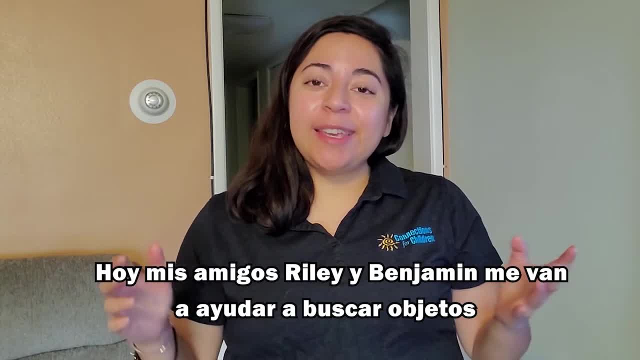 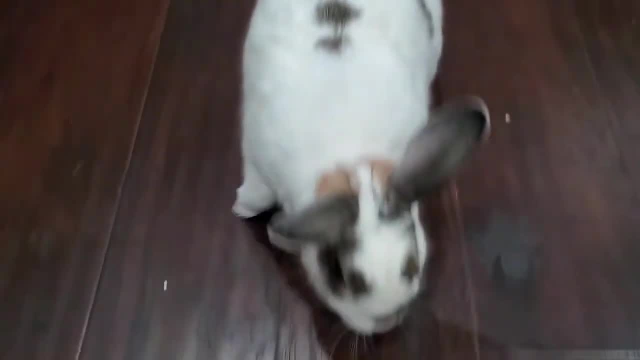 Hoy mis amigos Riley y Benjamin me van a ayudar a buscar objetos y vamos a rimar juntos. Benjamin, What rhymes with全部ial Three Bunny? Can you help me look for something that rhymes with bunny? Can you spot something? 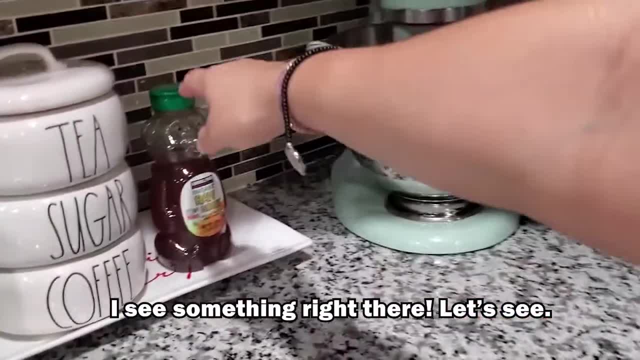 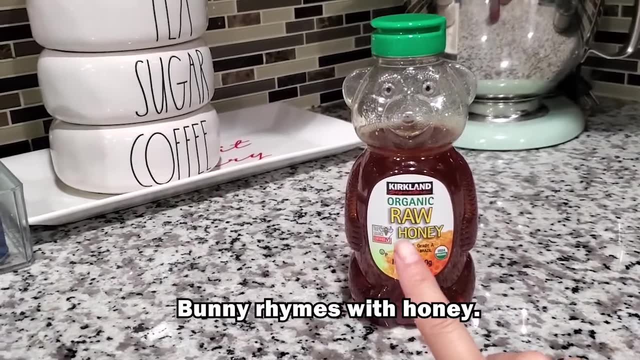 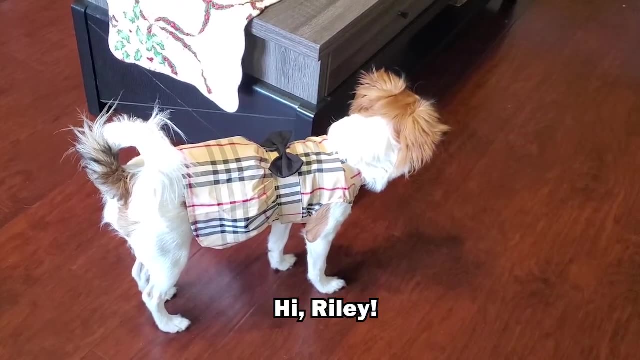 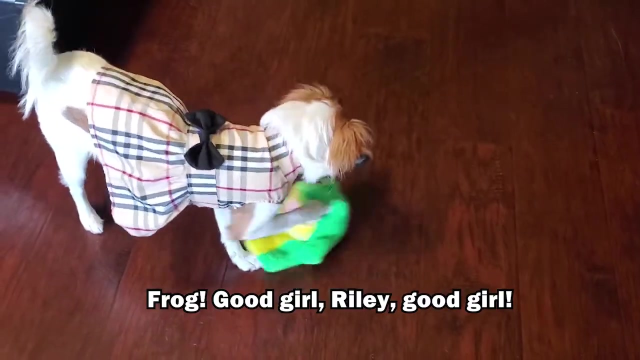 I see something right there. Let's see Bunny rhymes with honey. This is Riley. She is a dog. Hi, Riley, What rhymes with dog Frog. Good girl, Riley, Good girl. Dog rhymes with frog Perfect. 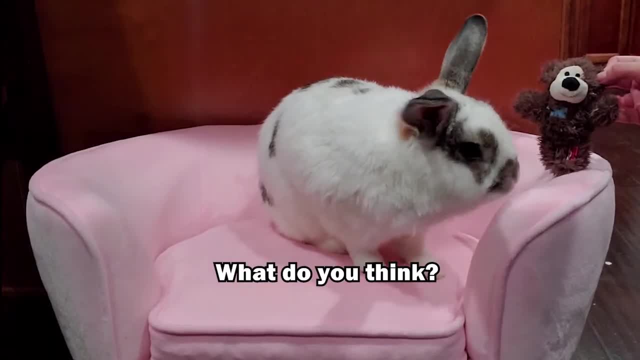 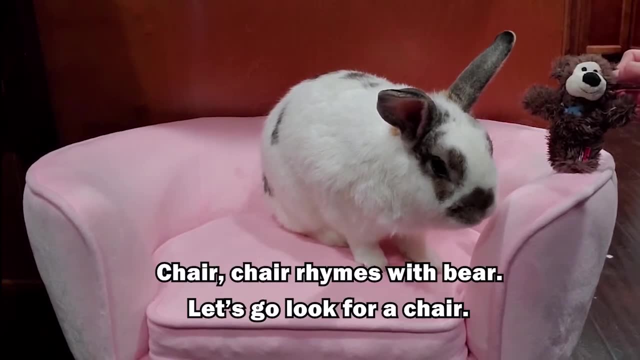 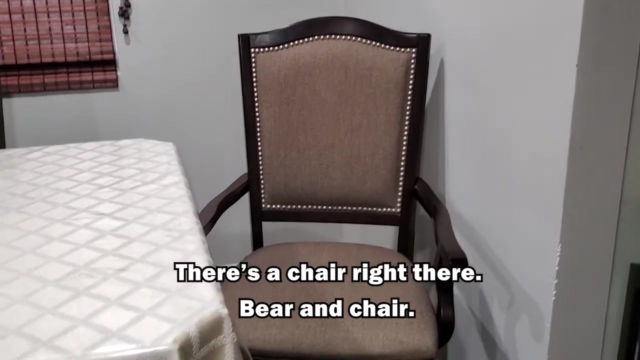 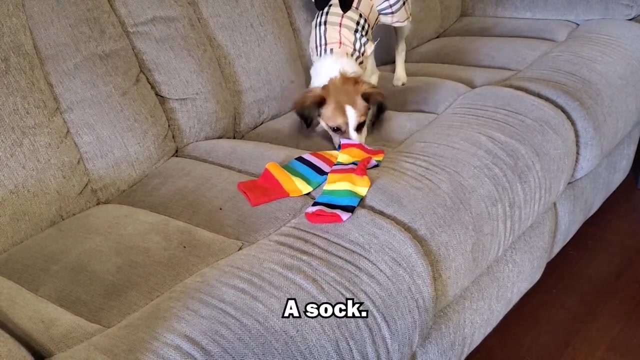 What rhymes with bear? What do you think, Bear? I know Chair, Chair rhymes with bear. Let's go look for a chair. There's a chair right there, Bear, and chair Riley. what do you have there? A sock. Can you help me look for something that rhymes with sock? 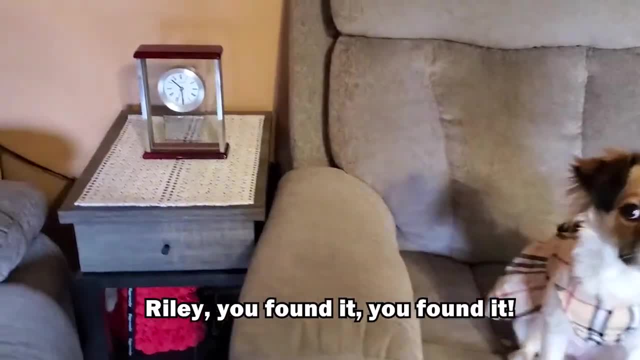 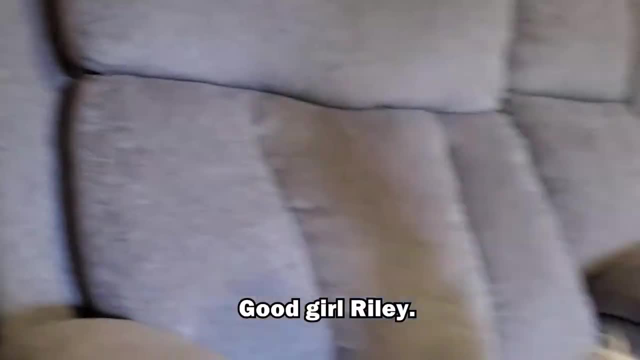 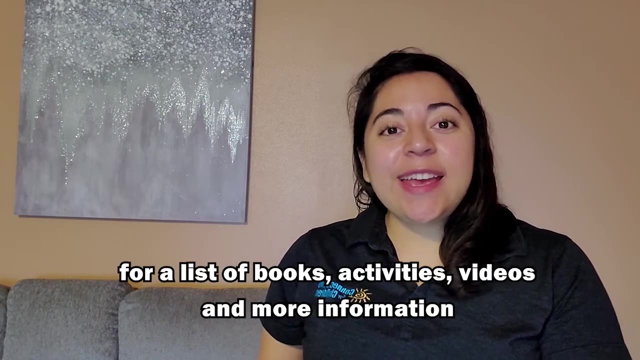 Hmm, We're looking, Riley, you found it. You found it Sock and clock. Good girl, Riley. For more resources, visit readingrocketsorg For a list of books, activities, videos and more information on how to support your child's early learning. 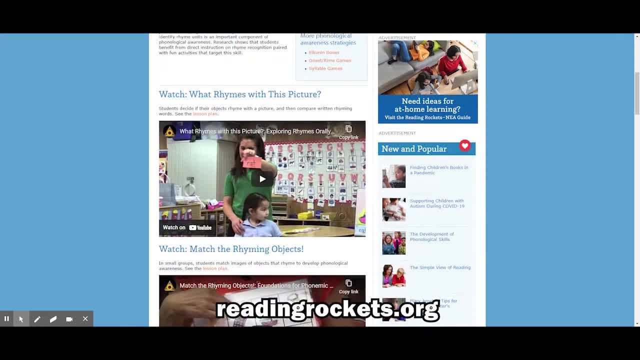 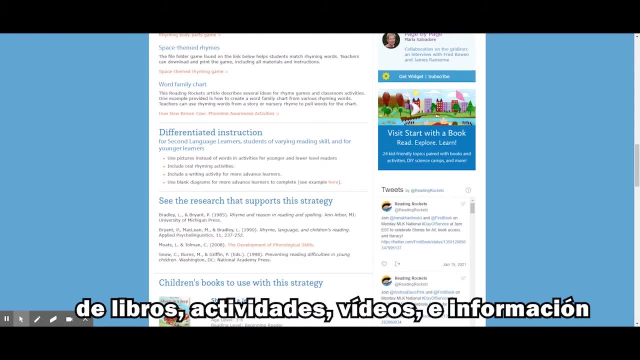 Para obtener más recursos. visite la página readingrocketsorg para más información sobre una lista de libros, actividades, videos y información en cómo puede ayudar el aprendizaje temprano de su hijo o hija. Today's tip is about early learning. 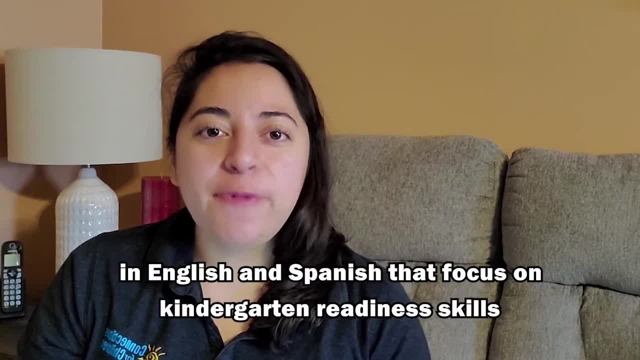 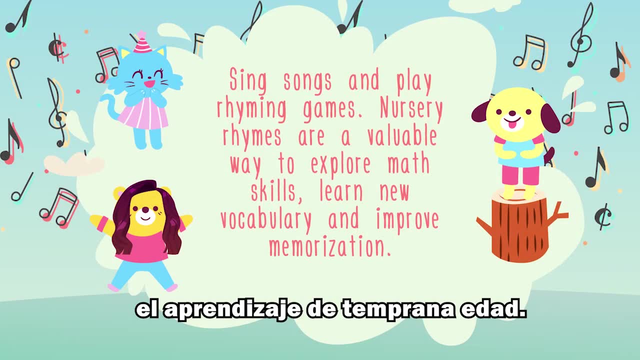 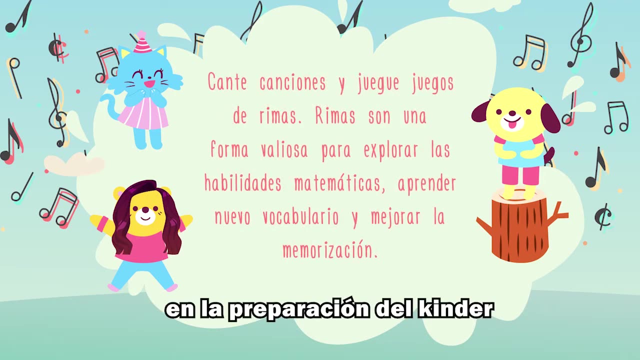 Building blocks are short video segments in English and Spanish that focus on kindergarten readiness skills through interactive activities. El consejo de hoy fue sobre el aprendizaje de temprana edad. Los cimientos son segmentos de videos bilingües en inglés y en español que se enfocan en la preparación del kinder a través de actividades interactivas y lectura.